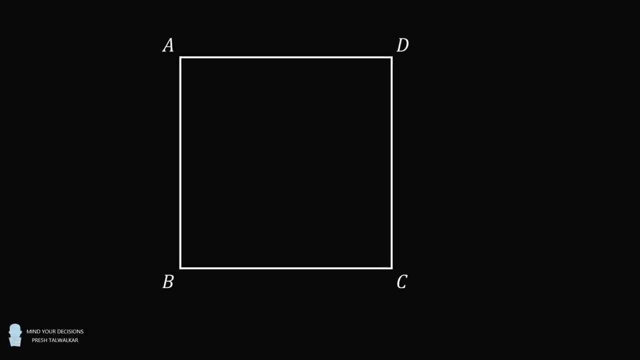 Hey, this is Presh Talwalkar. ABCD is a square. Construct the point M alongside AB, the point N alongside BC, Then construct AN DM, DN and CM. Let P be the intersection of AN with DM, Let Q be the intersection of AN with CM and let R be the intersection of CM with DN. 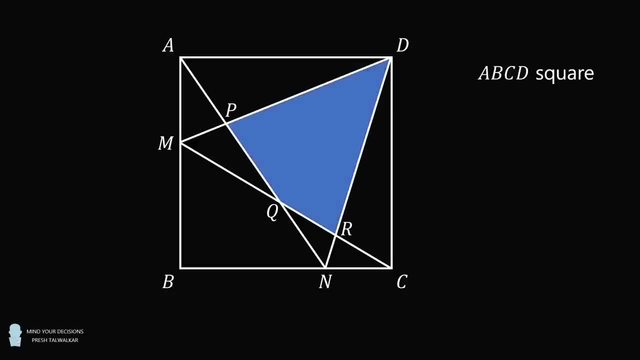 Consider one region, PQRD, that's shaded in blue. Then consider three regions that are shaded in green. These are the sum of the areas of APM, MQNB and NRC. The question is if the area shaded in blue is equal to 1,. 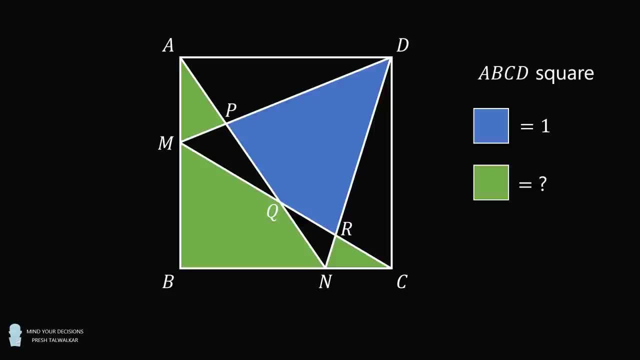 what is the total area of the regions shaded in green? I saw this problem via the website Cut The Knot, Pause the video if you'd like to give this problem a try and, when you're ready, keep watching to learn how to solve this problem. 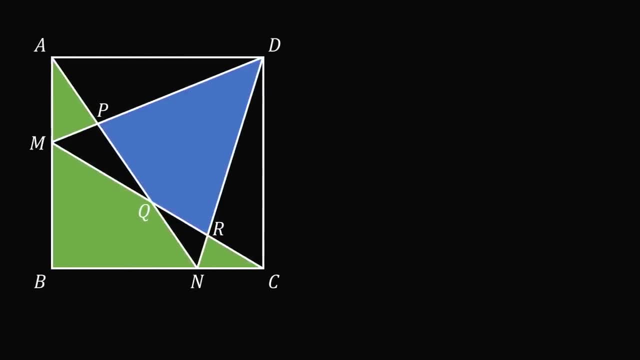 Let's first focus on the area that's shaded in blue. We want the area of PQRD. We will consider the triangle ADN. We can then find the area of PQRD by subtracting the areas of triangle ADP and NQR from triangle ADN. 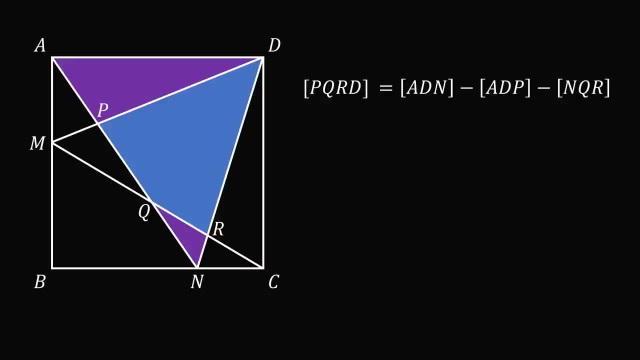 So now let's calculate the area of triangle ADN. Its area is equal to AD multiplied by a tight AB all over 2.. But AD is the ISO不對 on mT2.. Sometimes, when you remove the below area of ADN, the area of ADN is the same. 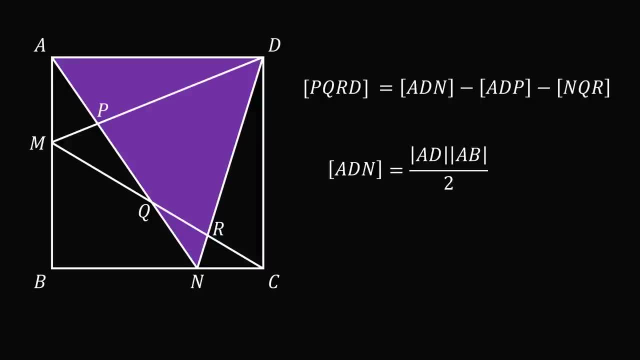 times AB is equal to the area of the square ABCD. So this is equal to the area of ABCD all over 2.. We can substitute this for the area of ADN. We now have an equation for the area of the region PQRD. 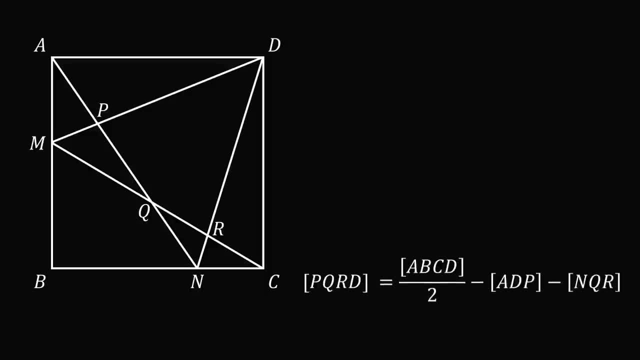 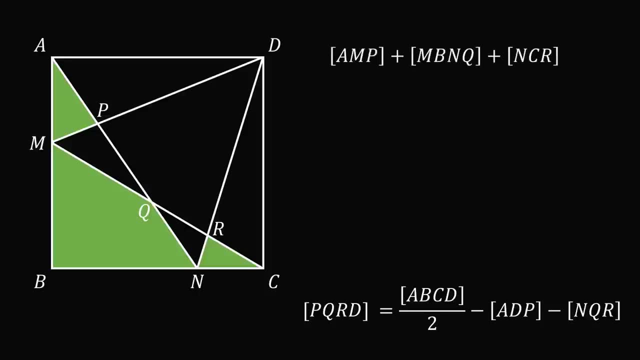 Let's now put this equation to the side and focus on the areas of the region shaded in green. We want to calculate the total area of the following three regions. We will consider the area in a different fashion. We'll consider the sum of the areas of triangles, ADM and MBC. 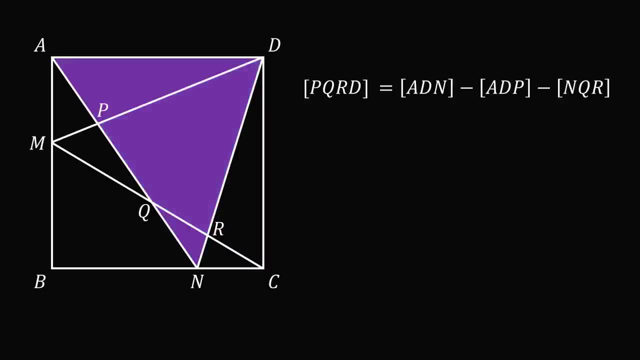 So now let's calculate the area of triangle ADN. It's area is equal to AD multiplied by its height, AB, all over 2.. But AD times AB is equal to the area of the square ABCD. So this is equal to the area of ABCD all over 2.. 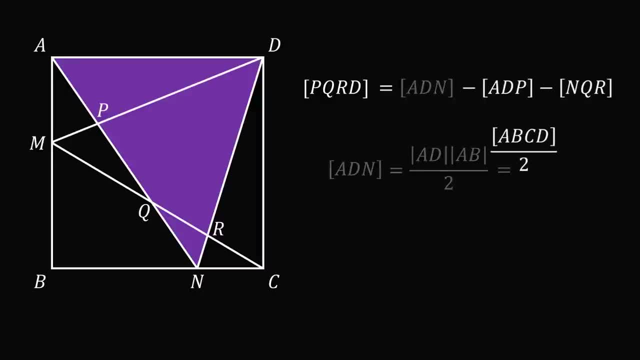 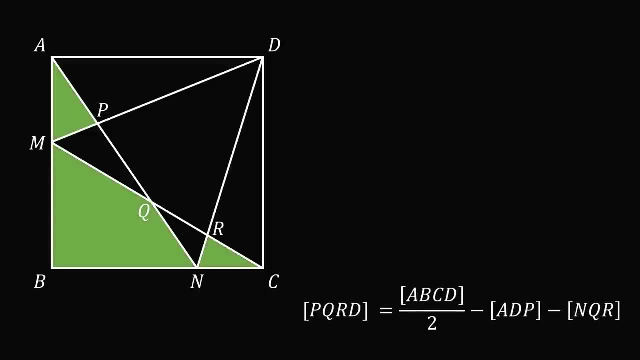 We can substitute this for the area of ADN. We now have an equation for the area of the region PQRD. Let's now put this equation to the side and focus on the areas of the region shaded in green. We want to calculate the total area of the following three regions: 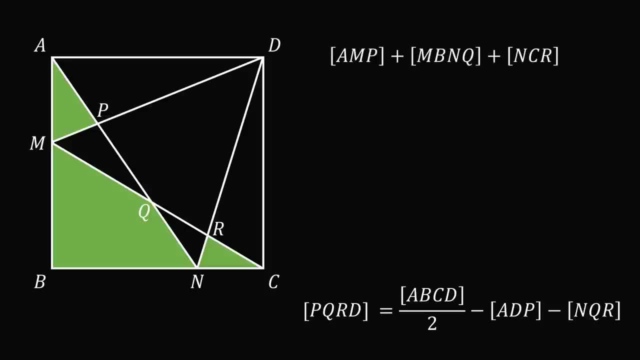 We will consider the area in a different fashion. We'll consider the sum of the areas of triangles ADM and MBC and then we'll subtract out the areas of the triangles ADP and NQR. This will be equivalent to the total areas that are shaded in green. 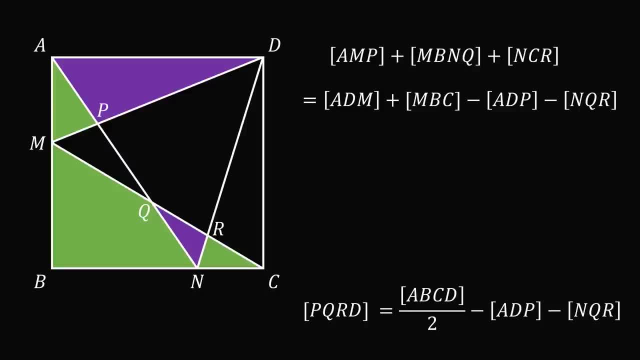 Now let's calculate the areas of the triangles ADM and MBC. The area of triangle ADM is equal to AD multiplied by AM all over 2, and the area of triangle MBC is equal to AD multiplied by MB all over 2.. We can now factor and we end up with AD multiplied by the quantity AM plus MB all over 2.. 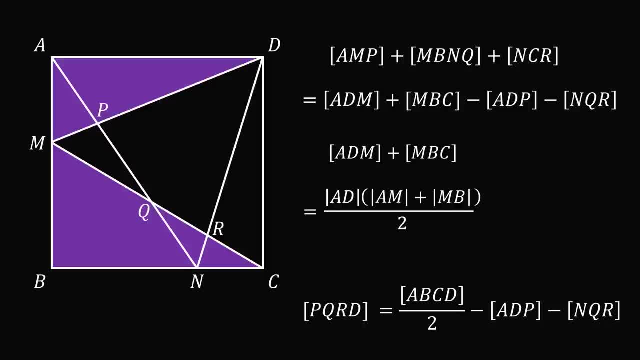 But AM plus MB is exactly equal to the length of AB. Okay, Okay, So the sum of the areas of these two triangles is equal to AD multiplied by AB all over 2, but AD multiplied by AB is equal to the area of the square ABCD. 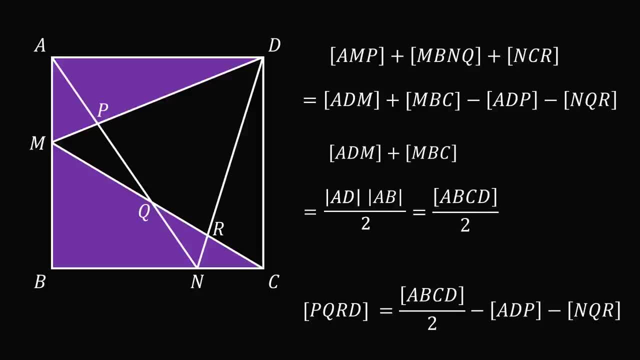 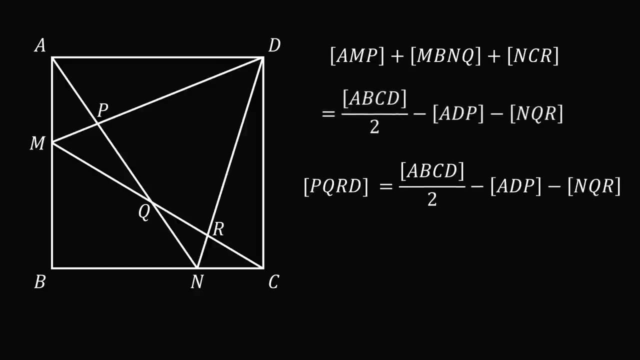 So the sum of the areas of these two triangles is exactly equal to half the area of the square. So we'll substitute that in for the areas of ADM plus MBC. We now have equations for the areas that are shaded in green. Okay. 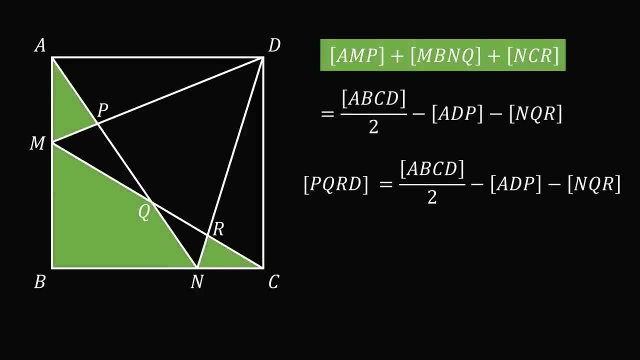 So we'll substitute that in for the areas that are shaded in green. That's the first equation And the area that's shaded in blue. We'll see both of these are equal to half the area of the square minus the area of ADP.